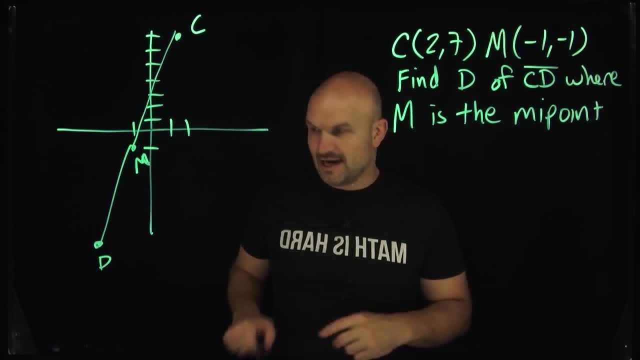 what's something that's kind of important or what's something that I think a lot of like I can take away from this that I could use. Well, one thing I would say- and this is a great way to like check your answers, This is a great like way to kind of foreshadow. 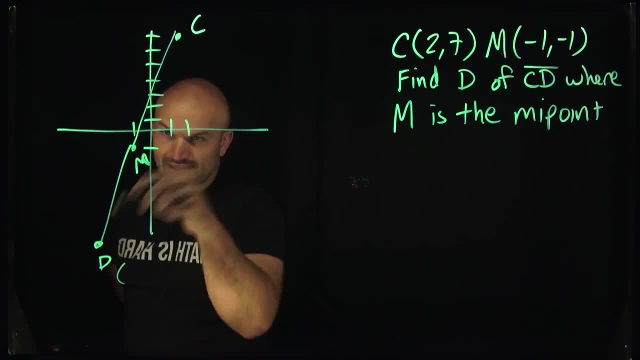 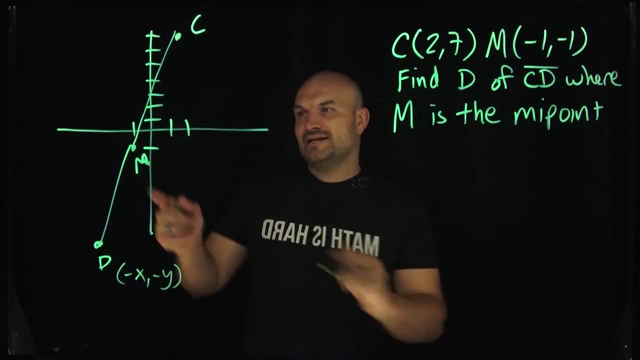 this: If you're taking a task or a quiz, I know in this coordinate or in this third quadrant, negative X and negative Y is my answer. So if I don't have a negative for my X and my Y, I know I did something wrong. right, Because it doesn't make sense for your. 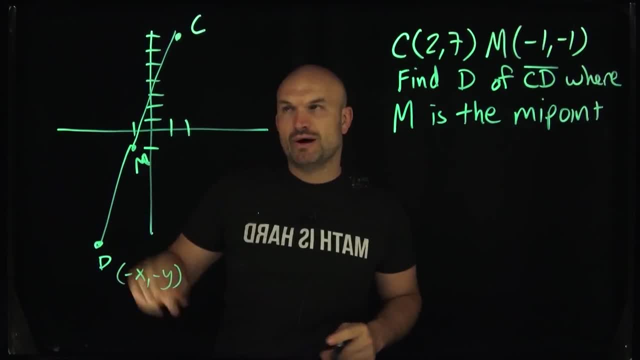 end point to be over here, right Over here. over here, It has to be down in the third quadrant, All right, So what do we know about these values? Now, I don't want to confuse you here with these negative X and negative Y. We're still going to treat this, We just 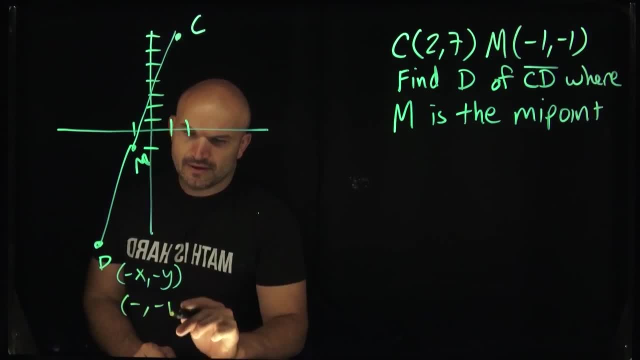 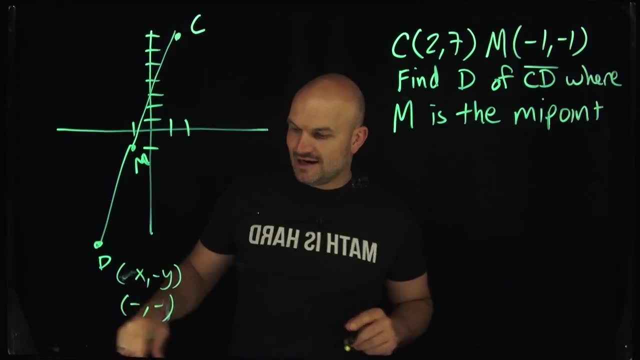 know these values. These values need to be negative. And actually let me just kind of maybe do this: We know the value, Oh sorry. We know the values are going to be negative. So I'm just going to kind of do that because I want you to understand this, that I don't know what these values. 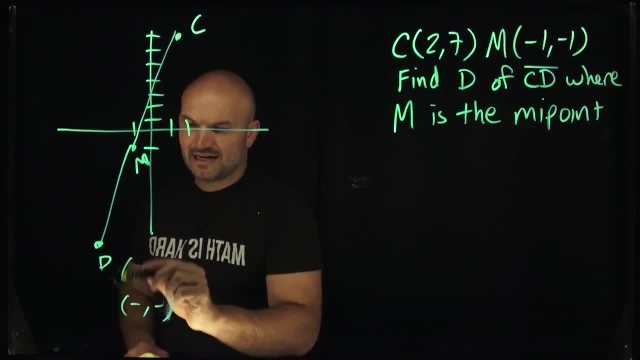 are. So I don't want to put the negatives here, because for the formula that we're going to use, that's not going to be helpful. So I'm just going to use an XY. All right, Now, even further than that, what I'm going to do is actually, I'm going to call these X3. 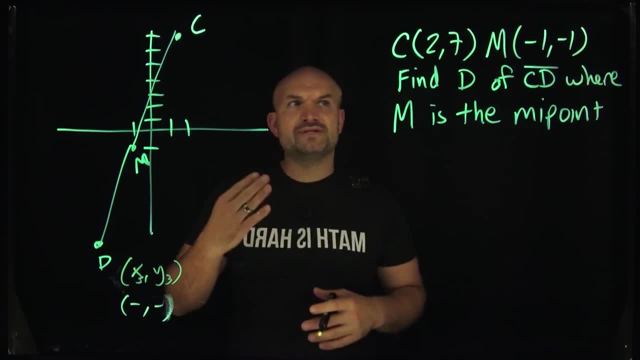 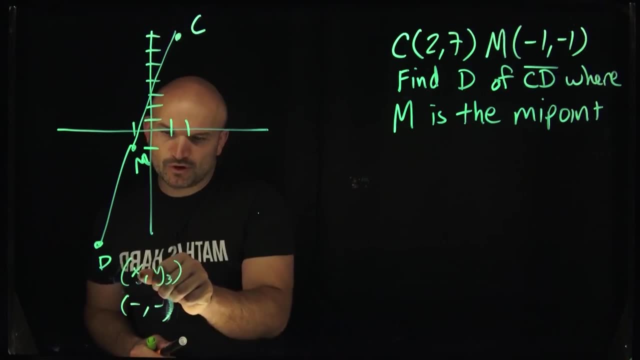 and Y3. Because, if you remember, in the traditional, like midpoint formula, we use X1 and X2 as those two coordinate points. We are going to use these as X1 and X2.. Sorry, Because the coordinate points, if you remember, was always going to be a X2. 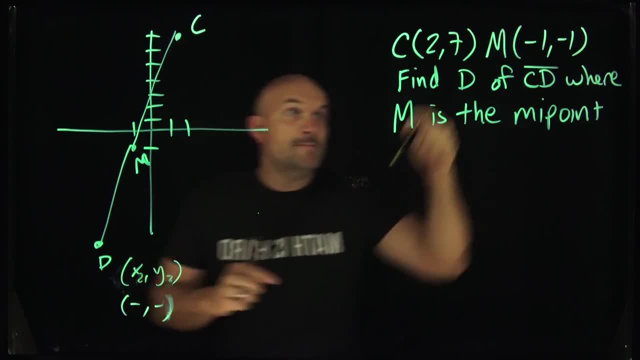 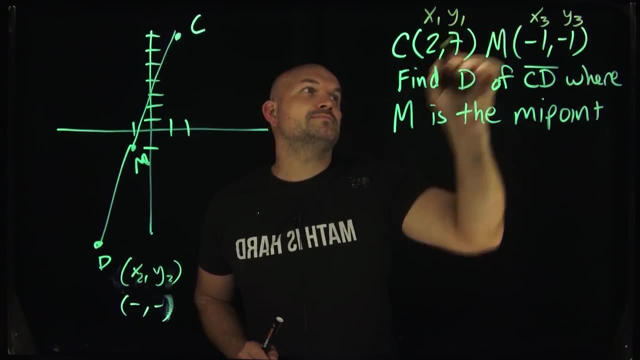 and a X3.. There we go Now the midpoint, though. we're going to call these an X3 and a Y3.. And we'll call this an X1 and a Y1.. Okay, So remember, midpoint formula, right What? 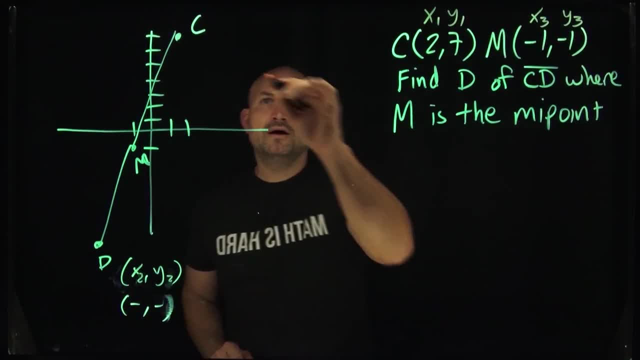 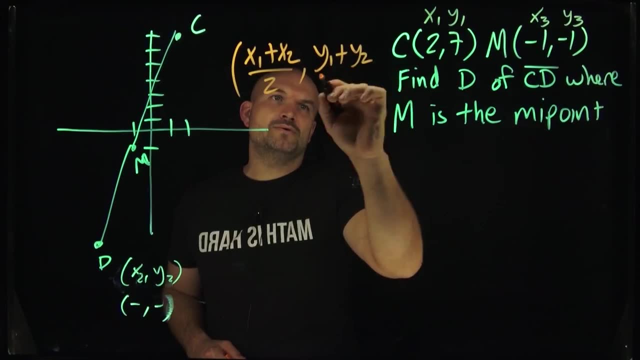 was the midpoint formula. Well, if you remember, the midpoint formula was simply, you know, X1 plus X2 divided by X3. And then a Y1 plus a Y2 divided by 2.. Right Now again, what those gave us was 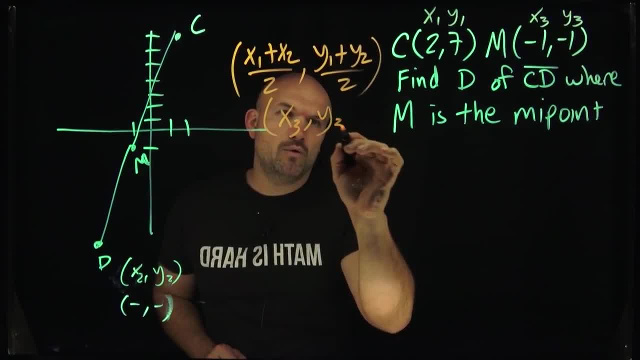 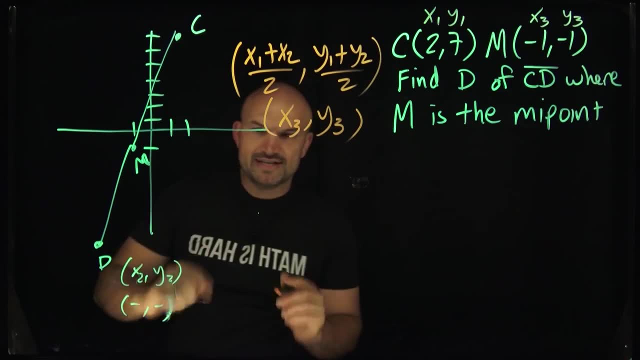 our midpoint, which I'm going to call X3 comma Y3.. Now, why would I call them that? Why would I do that? Well, the reason why I would do that, guys, is because I want you to understand this. If we were to kind of like write an equation here, I can say: X1 plus X2 divided. 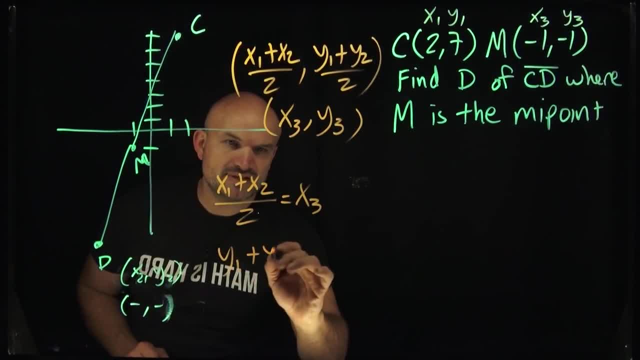 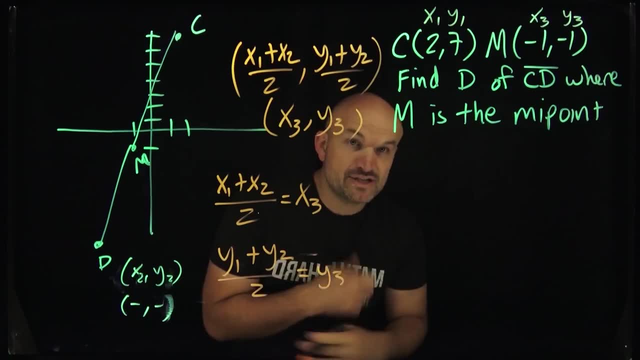 by 2 equals an X3.. I can also say: Y1 plus a Y2 divided by 2 gives us a Y3.. Right, So now we need to understand well what is the information that we have and what is the information. 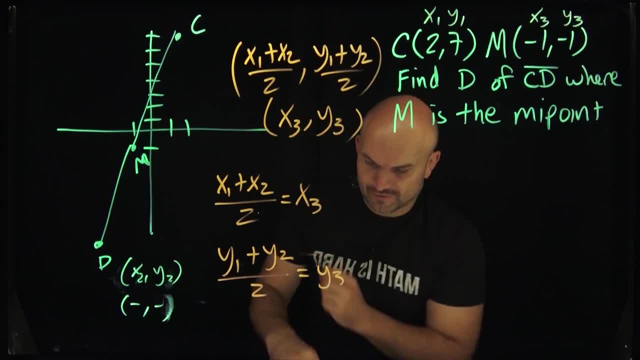 that we don't have. So if we look at this original problem or the original information we have, we say, all right, do I have an X1? Yes, that's 2.. Do I have an X2? No, I don't. 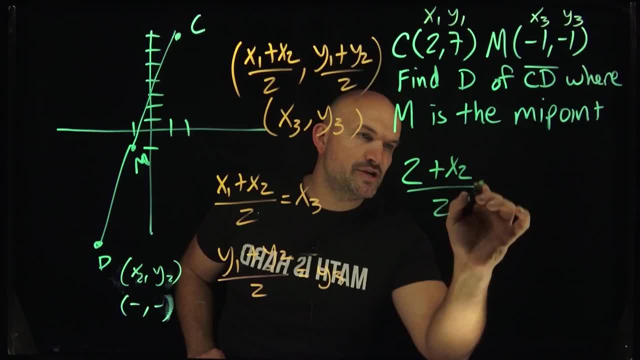 know what the X2 is right. So it's going to be plus an X2 divided by 2, and that equals X3.. Do I know what X3 is? Yes, I do. That's a negative 1.. Okay. 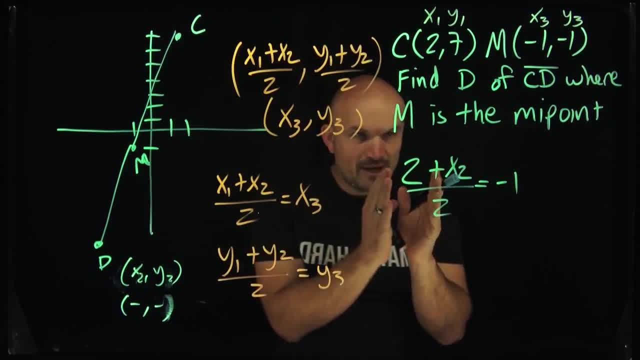 Now how can I go ahead? and you know, solve from here. So again, remember when you're dividing by 2, if you want to undo dividing by 2, you just need to multiply by 2 as well. 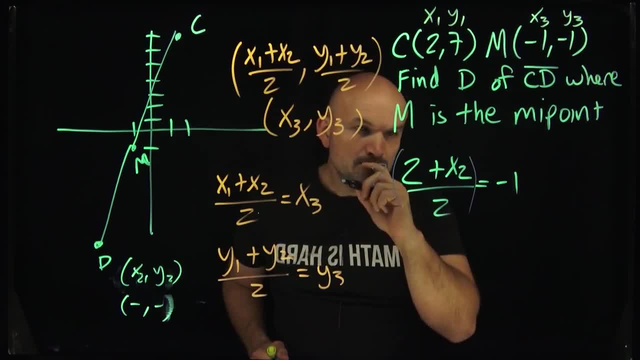 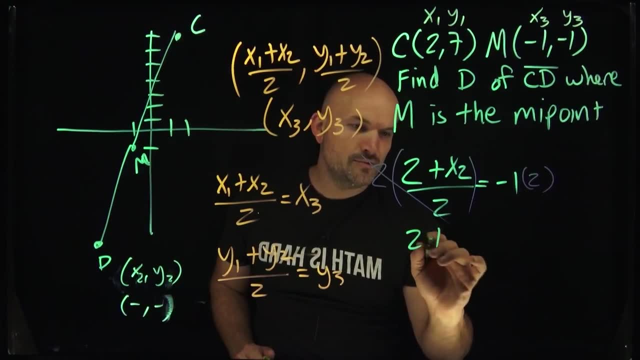 Now. what I'm going to do, though, is I'm going to put everything in parentheses here, So, therefore, you can see that those are going to multiply out, and then you multiply by 2 over here. Then what you're now going to have is a 2 plus a X2 equals a negative 2. Now, 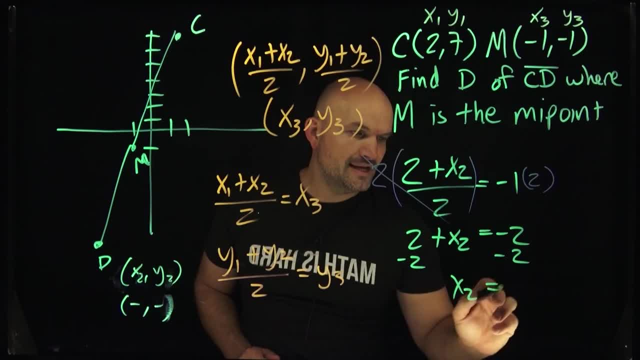 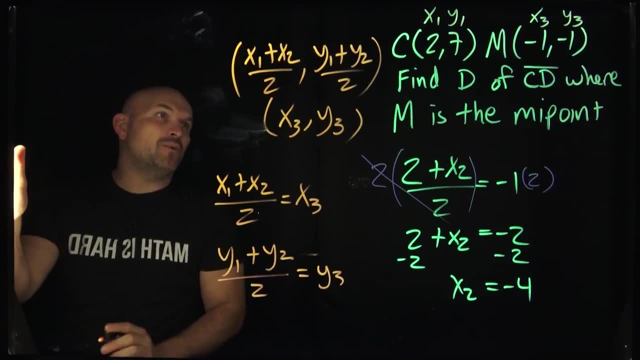 I can subtract the 2 on both sides and I get a X2 is equal to a negative 4.. All right, I wasn't really planning on using that much space, but we'll do this again. Now let's do the Y. So do we have a Y1?? We do have Y1. That's going to be a negative 4.. All right, 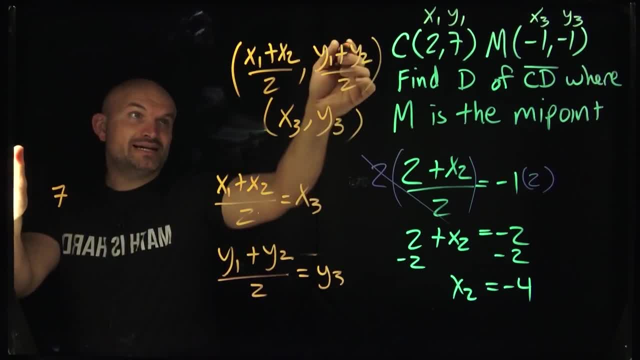 A 7 plus Y2, which we do not have. right, The Y2 is our unknown. That is going to be our second point, So it's going to be: plus a Y2 divided by 2 equals a Y3, which we do. 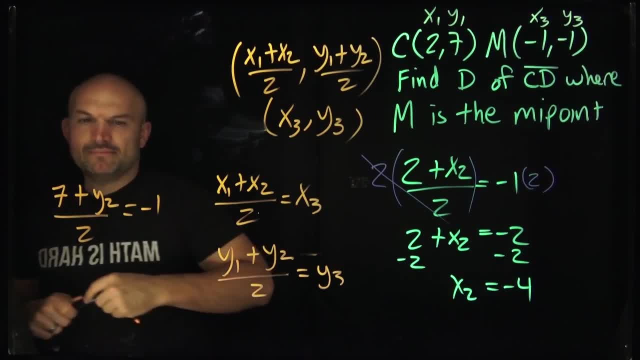 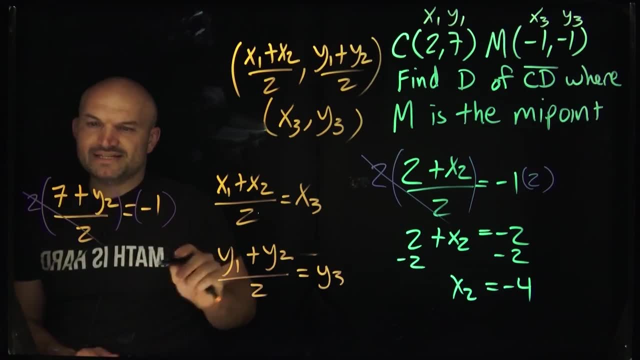 know what Y3 is. That's going to be a negative 1.. So again, I'm going to go ahead and multiply by 2 on both sides. Use parentheses, because you're multiplying everything by 2, right, And you can even do the parentheses over here if you want to, But these now are going to. 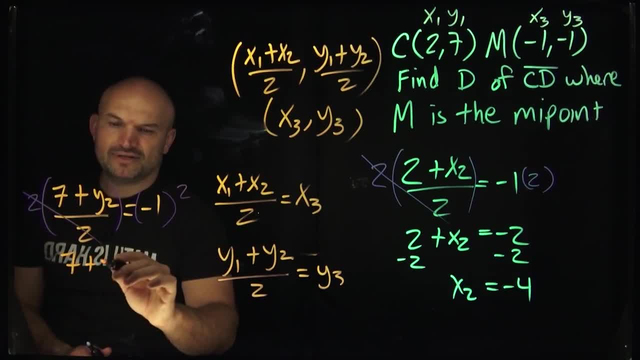 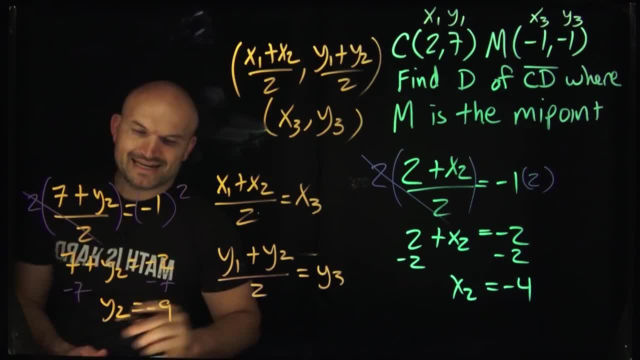 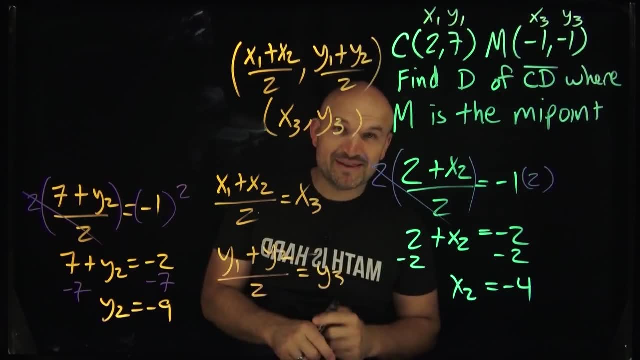 the 7. Y2 is equal to a negative 9.. So, therefore, the other endpoint is now going to be a negative 4, negative 9, which, if you remember, was supposed to be in the third quadrant Is this: 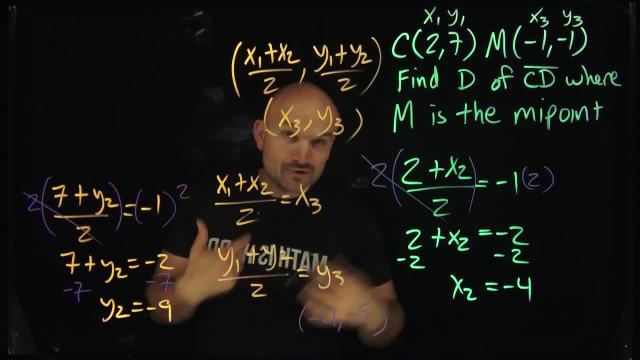 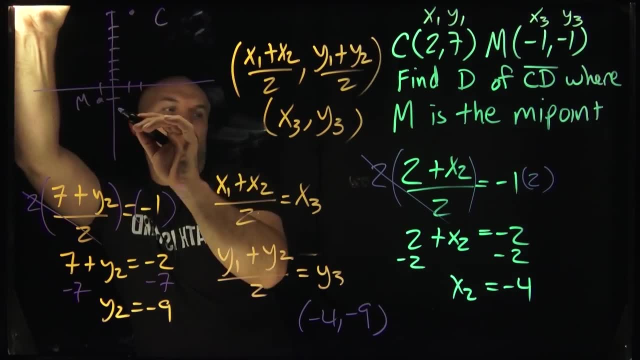 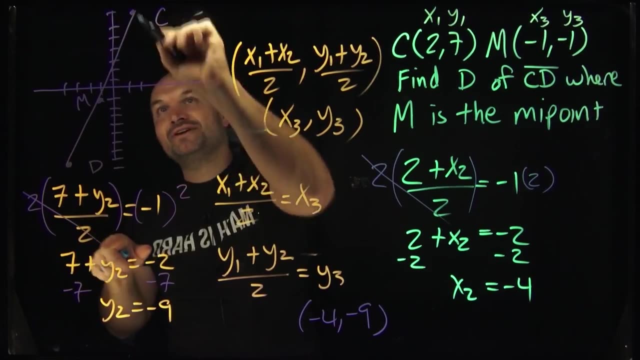 coordinate point: negative 4, comma, negative 9? Is that going to be in the fourth quadrant? Yes, it is. Let me just go ahead and scratch this up real quick. There we go. You can see, does that look like I did a pretty good job. 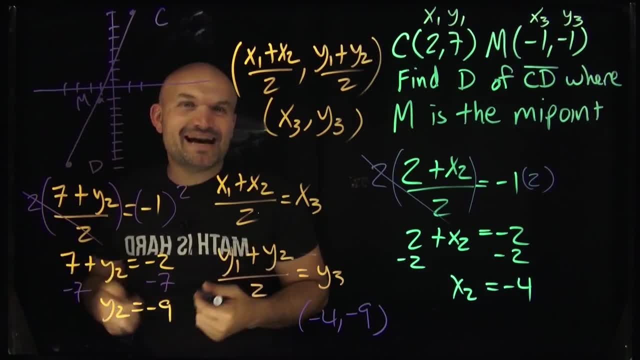 I mean I had to erase my original graph, but you guys can see like I think that's a pretty good job. So thankfully we can rely, we can use this graph to make sure that we're getting our answer correct. But in the next video we'll go ahead and explore to. 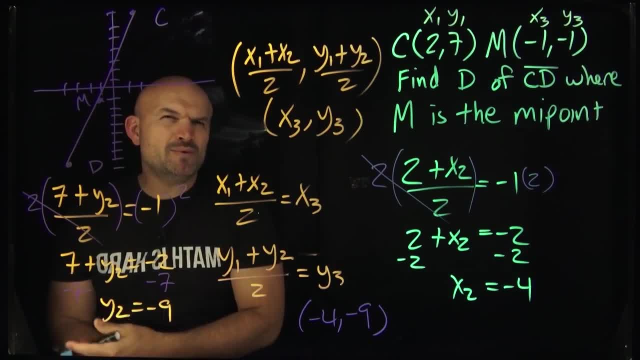 visually verify our answer using the graphical approach. But what about when we can't verify the midpoint using the graphical approach? That will come up in the next video. We've seen the trend all through this season with clubs charging away fans an incredible amount of money. Clubs know that we will always fill our capacity. Our people will pay whatever it needs to get to it, but we expect to be treated fairly. We don't ask UEFA to go and see the airlines and ask them to give free prizes to our fans, but to have an impact on where they actually can make a difference. 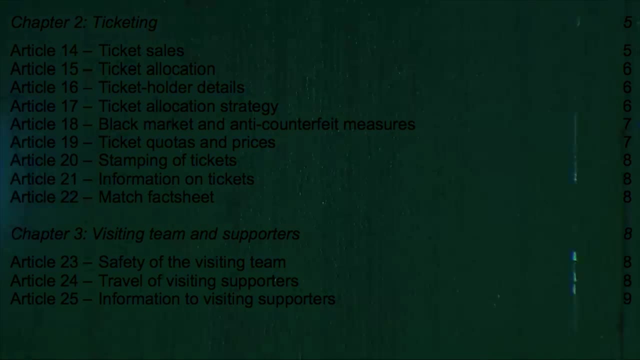 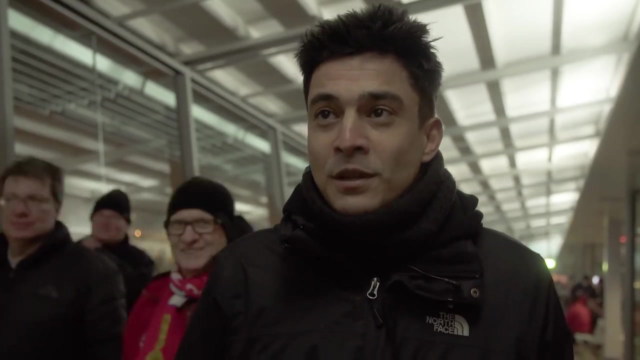 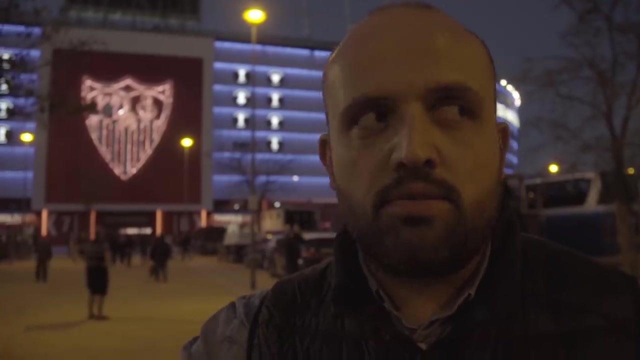 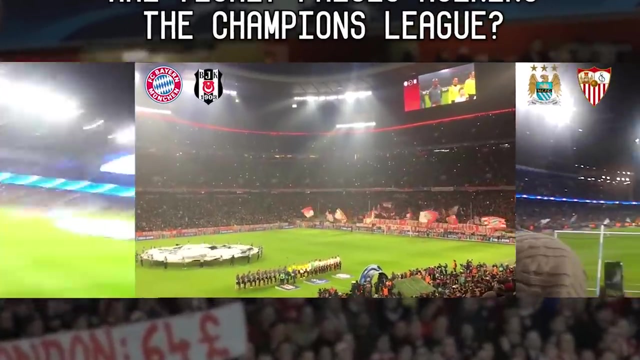 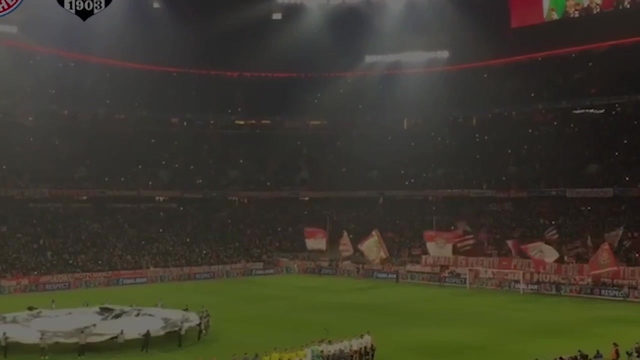 We are the people who really come for the game, for friendship, for supporting, and we pay for it. The rest of the people always earn out of it. This happened in the past, but there is an accumulation of those situations. What's up, Copa fan? We're in Munich, Germany. We're doing a little exploration right now on fan rights when it comes to attending European matches. 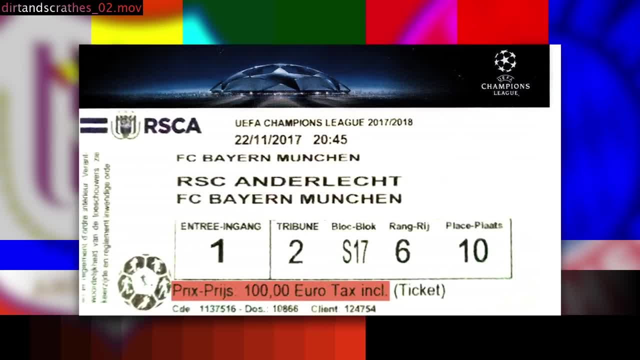 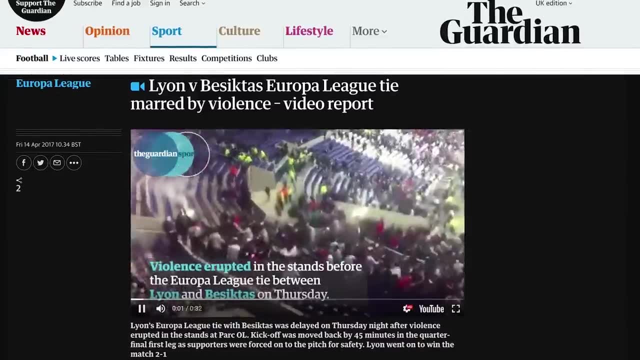 So last year Eindrallach- the club- charged Bayern Munich fans too much money and UEFA went back and had them actually reimburse Bayern Munich fans. This year, Besiktas fans aren't being allowed to attend the Bayern Munich game because of some issues with the clubs not taking responsibility over fan management. 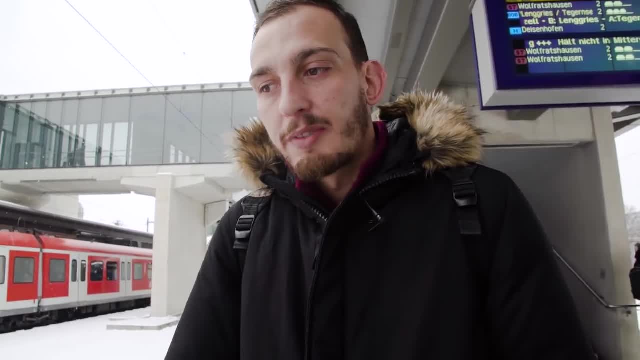 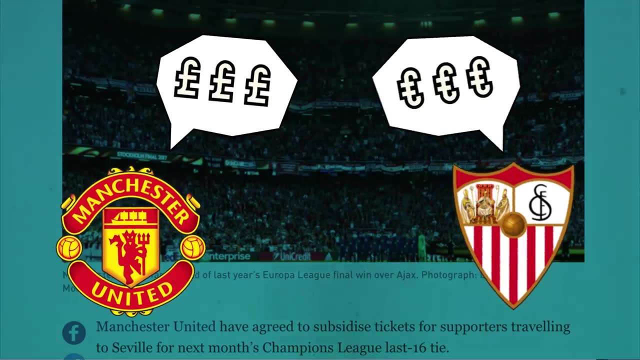 Tomorrow we head off to Seville, where Seville is playing Manchester United, and both clubs have actually had to subsidize payment for tickets for their fans to actually raise the prices. Now, the thing to call into question here is that football clubs are no longer a responsible body. 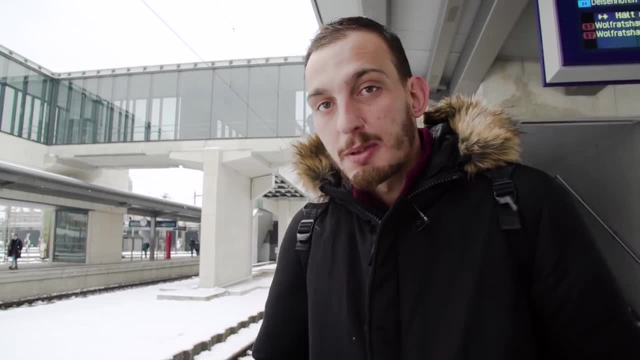 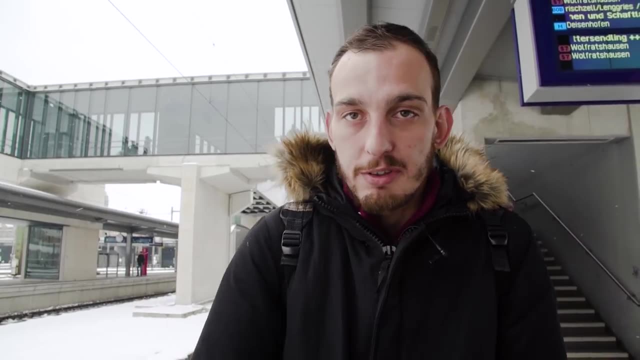 Unless they're regulated, they'll keep trying to profit as much and much as possible, and that becomes particularly evident within the European football scene. We're going to speak with football supporters in Europe: supporters of Besiktas, Bayern Munich, Seville and Manchester United. 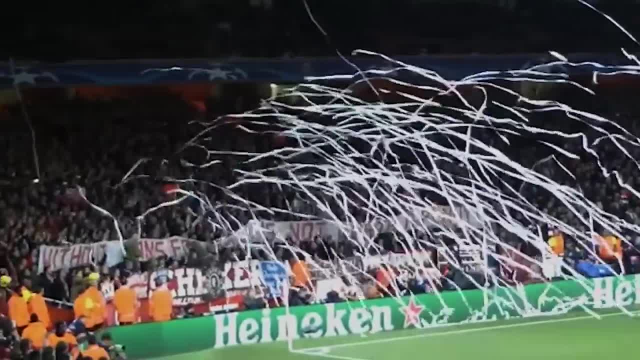 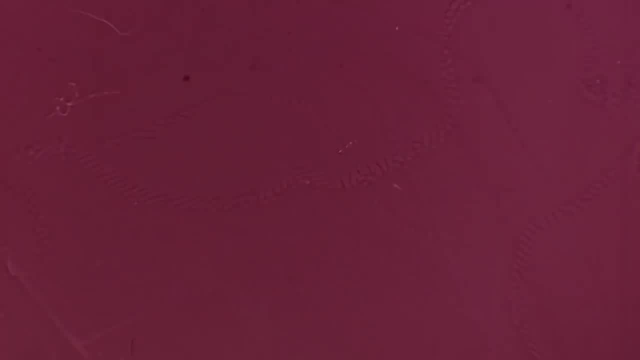 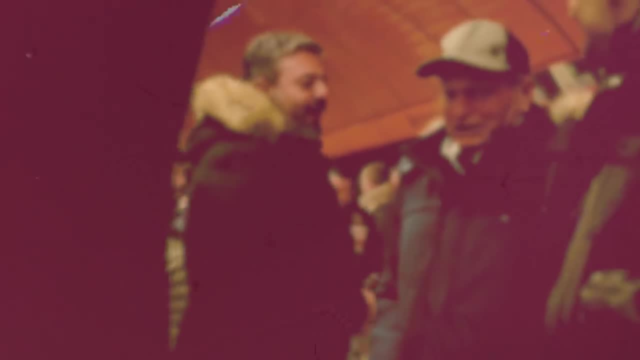 all about some of the struggles that fans in European competitions regularly face and why fans are being taken away from the most special and exciting competition they could possibly attend. Tonight you see guys singing Besiktas chants behind us wearing Bayern Munich hats.